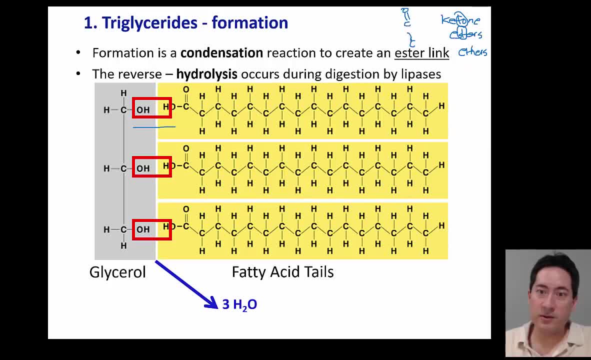 I remember those. Those have the O sticking out of nowhere, And so the ethers are the ones with the O in the middle, And the ketones are the basic starters, And then, as we learn more, esters are the more complicated. 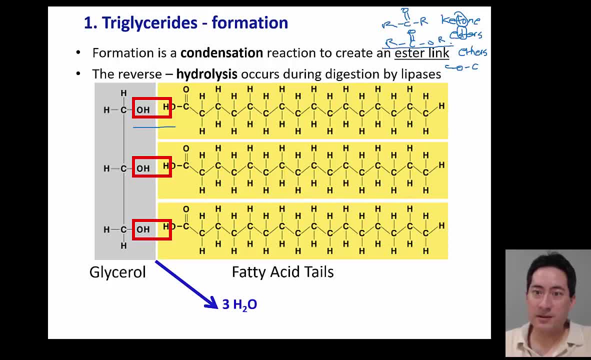 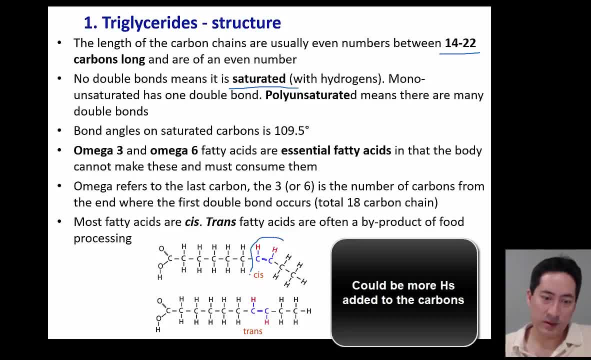 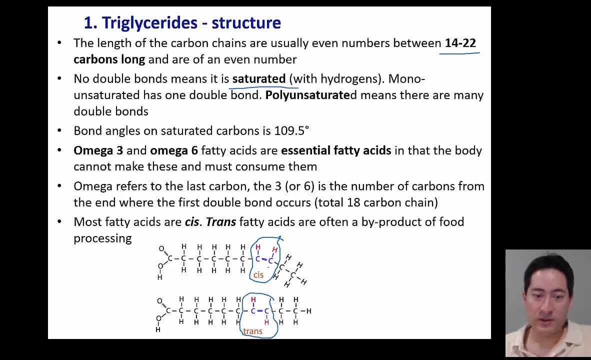 the last two, B1 and B2.. And so we've already talked about condensation and hydrolysis. quite a bit from saturated. your guide for standard levels says you don't need to know cis trans because that's high level. but I find it quite helpful to try and picture. why are trans so demonized and why? 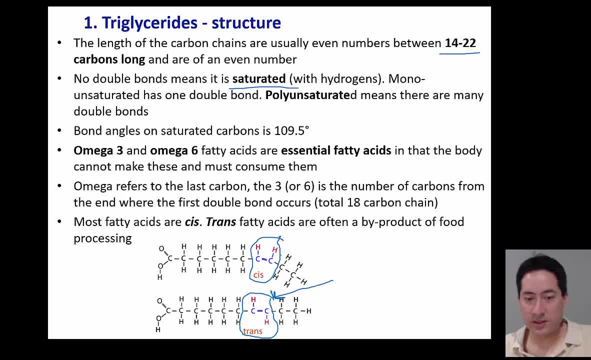 are they meant to cause so many health effects? I just kind of consider that- and this is sort of jumping the gun- saturated fats, because they are all saturated, they're all nice straight lines and they stick together and they have a high melting point and boiling point because they 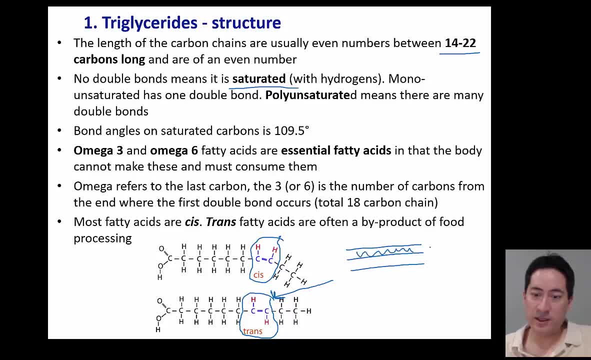 have a nice close surface area here, and so they have London dispersion forces sticking them together. Now saturated fats have this kink in them, so these things actually do go up and down slightly- if I had a 3D model out, but these kinks really do create these massive gaps and I just 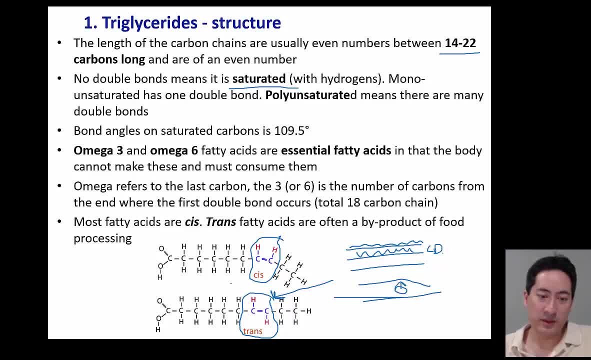 figured that the enzymes have more accessibility And if you look at cis, there's a huge gap here. and this is very electronegative and the trans not so much so. So, for the same reason, that's how I understand trans to be particularly bad and saturated to be particularly bad. 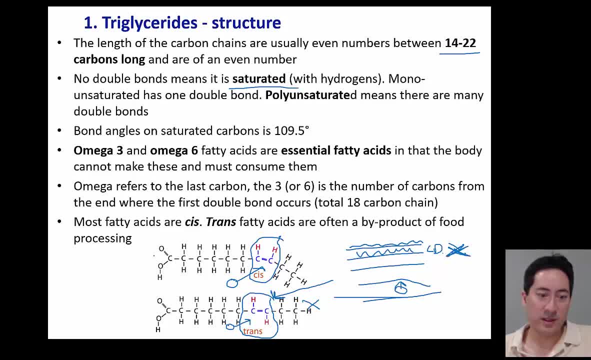 because it's already hard enough for the enzymes to access these fats. that's why we have bile salts to emulsify them into the water to get access, And being trans or being saturated just makes it that little bit more difficult still for the enzymes to get in there and break them up. 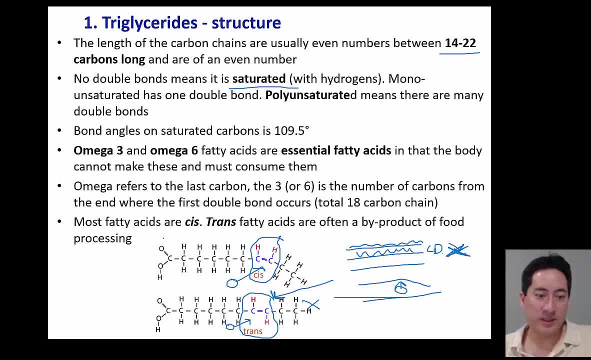 And so that's the chemical basis for my understanding of how I understand why they're good or bad for you, Just basically, whether or not enzymes can access them or not. Okay, so that's my take on all of these, The chemical structures and things like that. 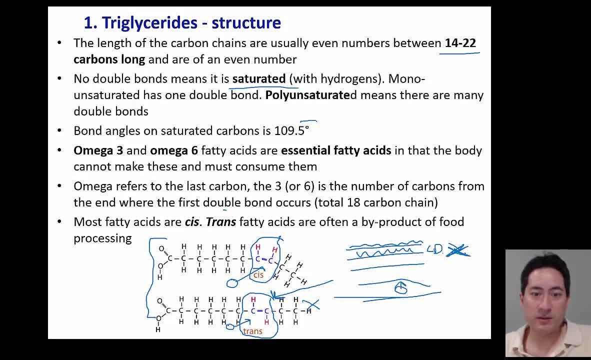 So I'm going to show you a little bit more detail there. So 109.5, that's tetrahedral. There are certain fatty acids we can't make, so omega-3 and 6. So that refers to three: the number of carbons from the land where the double bond occurs. 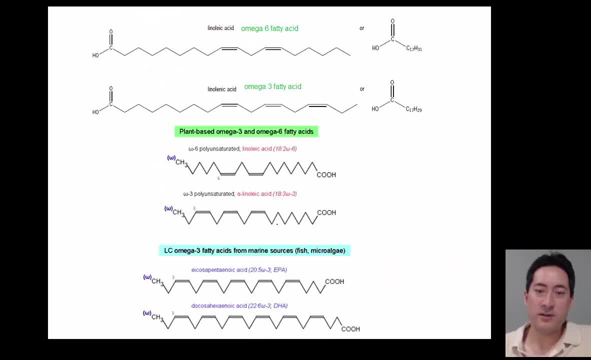 And so, just out of curiosity, I have got some of those. So that's the carbon on. third carbon on. there's a double bond there: One, two, three, four, five, six and a six, So that's omega-3 and omega-6. 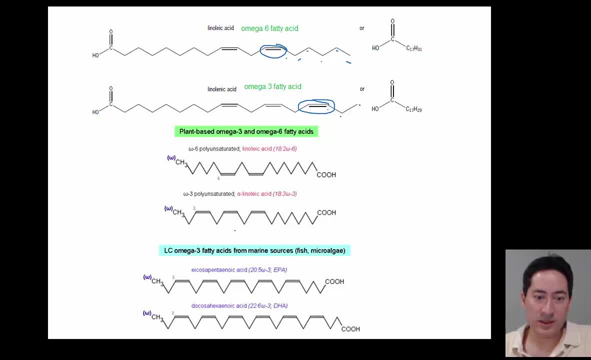 And, out of curiosity, the plant ones and animal ones and I guess the fish ones. they do look different. So there's also a bit of controversy out there about plant-based proteins and animal-based proteins. They're all different. They are actually chemically different. 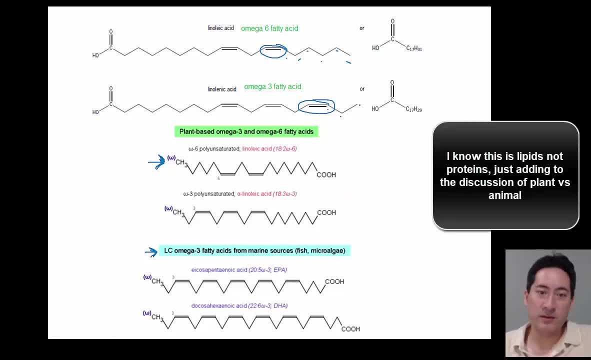 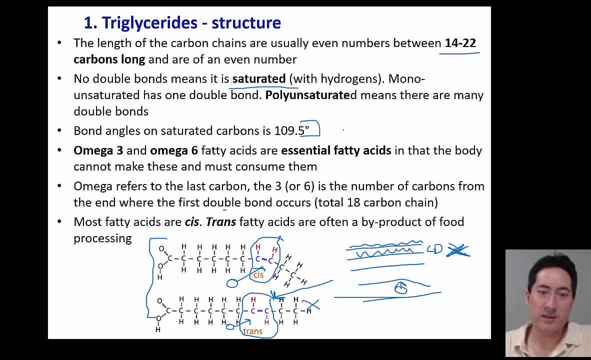 But they are omega-3, because that's what the definition of omega-3 is- is the third one from the end. This one's going in this direction. So that's three carbons along, that Six carbons along. Okay, so you could be asked details like that. 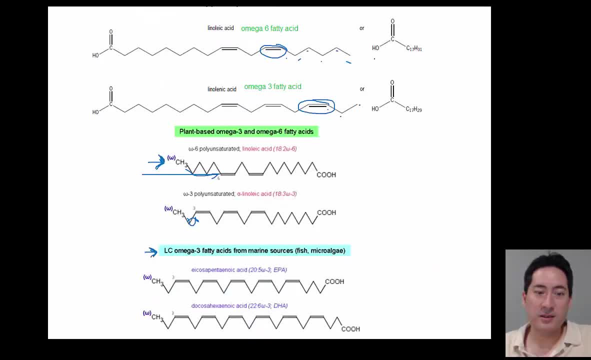 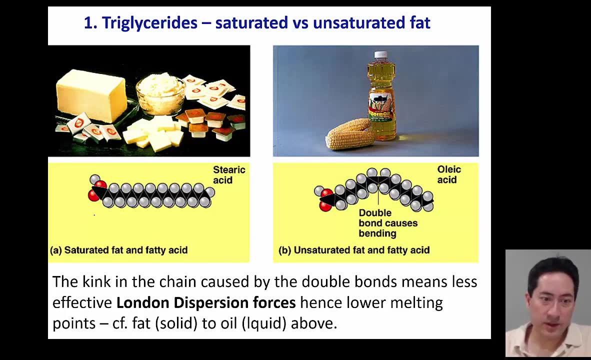 It would be unfortunate but you could be asked. So moving along. so, as I just mentioned in the previous slide, saturated versus unsaturated. So if there are lots of these molecules and they're nice and straight like this, there will be more London dispersion forces between them. 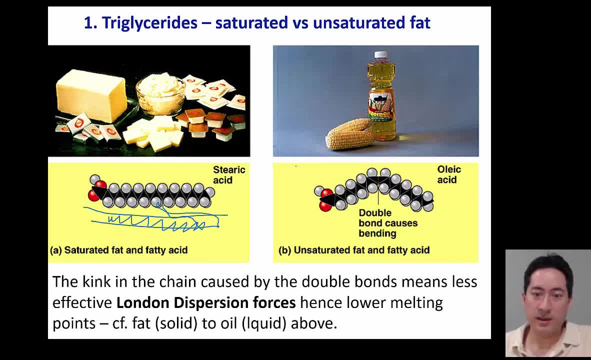 And so they will be more likely to be in the solid state And unsaturated fats. because they've got that kink, they don't have as much surface area and parts where they're sticking and lining up with each other, So they will more likely be liquids. 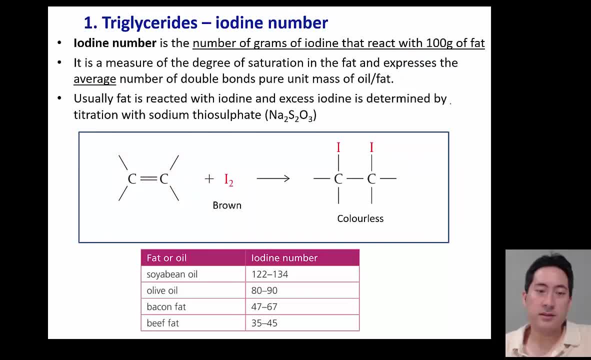 So the iodine number tells us exactly how saturated the fat is. So if the fat is very saturated, not much iodine will react. If it's unsaturated, then there will be lots of double bonds for the iodine to react in this fashion here. 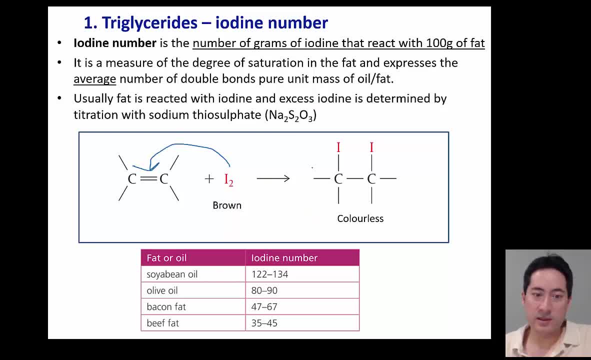 So the iodine will come into the double bond and it'll go from brown to being colorless in this reaction here. So we want unsaturated fat, So we want the iodine number to be high. So, if you look there, soybean and olive oil are famously touted in the media as good for you. 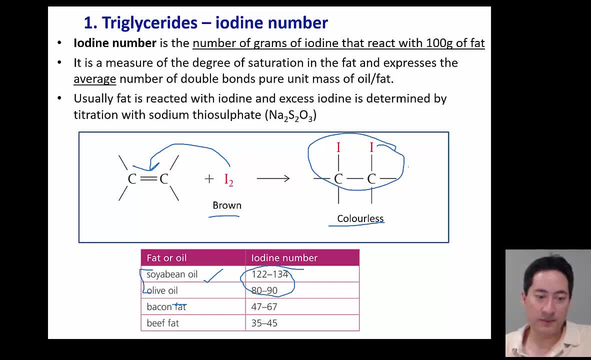 And they have very high iodine numbers, where animal fats are very saturated. You can see they've got very low iodine numbers here And so it's important to memorize this formula here. So it's important to memorize this definition here. 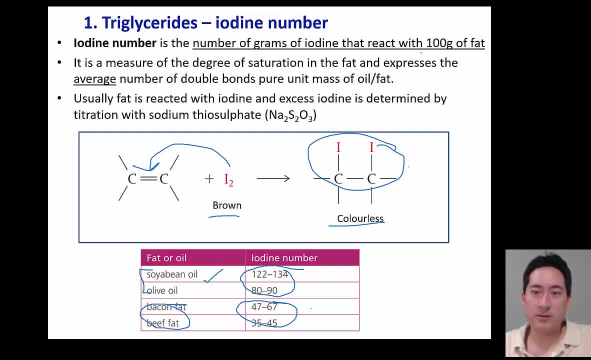 The iodine number is the number of grams of iodine that react with 100 grams of fat. So this is a titration where there's a two-step reaction to. by the way, So thiosulfate reacts with the excess iodine. 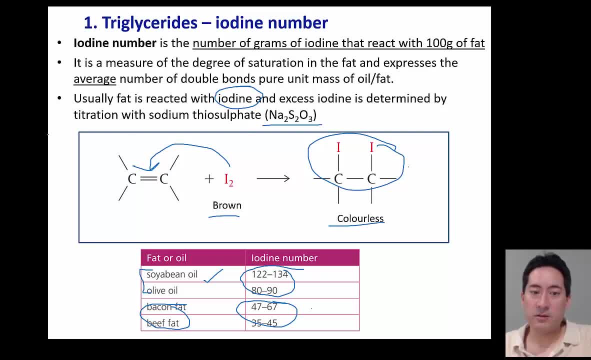 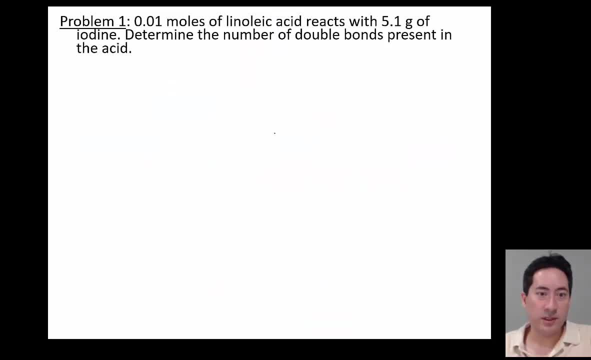 And that's how you do your calculations to work out how much what the iodine number is. So this is an example. So point three: So 0.1 moles of linoleic acid reacts with 5.1 grams of iodine. 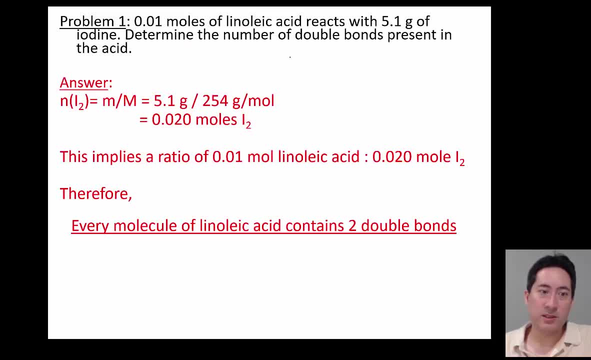 So how many double bonds are present? So first of all you work out how many moles of iodine has reacted. So if 0.02 moles of iodine has reacted, then and you've only had 0.1 moles of linoleic acid. 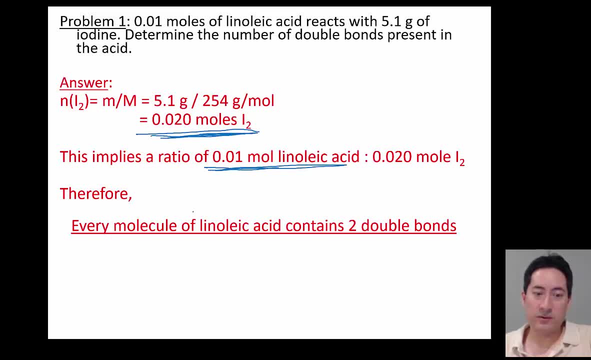 that means there was two double bonds for every molecule. So for every mole they needed two moles of iodine. So for every molecule of linoleic acid there was two molecules of iodine. That must mean there's two double bonds. 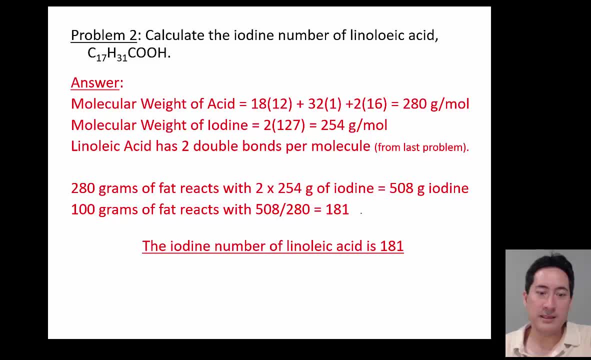 So the next question is just an extension of that. So what is the iodine number from that then? So calculate the iodine number of linoleic acid. So we need to work out the, the number of grams of iodine that reacts with 100 grams of fat. 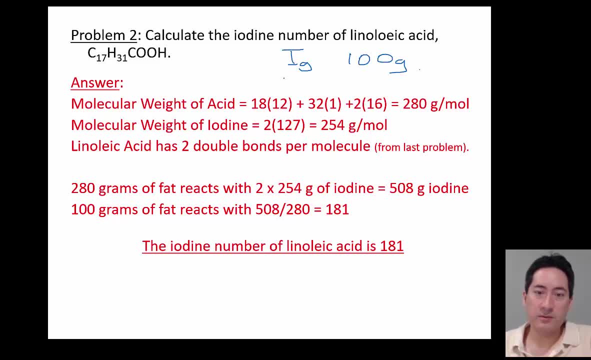 That's the definition, So what we have here. we need to work out how many moles is in 100 grams of fat, So the molecular weight of the linoleic acid. If you look at that formula here, we do that there. 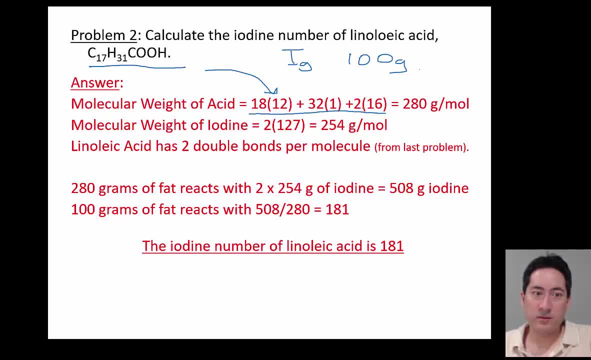 So there's two oxygens here and 32 hydrogens and 18 carbons, so we get 280 grams per mole. The iodine is I2, and so that's 254 grams per mole. Linoleic acid has two bonds per molecule. that we know from the last problem. 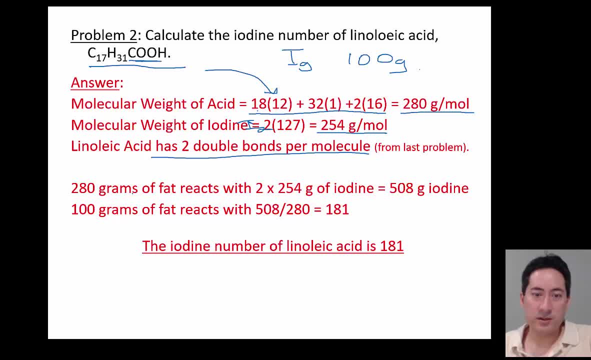 So basically, you just say that you had 280 grams and that's the ratio there: 280 to 254.. But we're not going to get 1 is to 1.. This is a 1 is to 2 reaction. 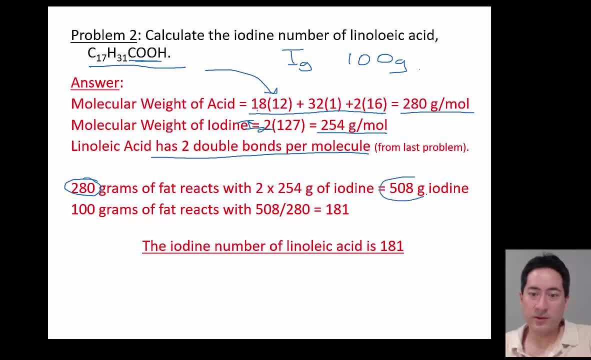 So if we have 280 grams, we're going to have 508 grams of iodine necessary. So this ratio here, 508 divided by 280, it's going to give you the number of grams of iodine per gram of fat. 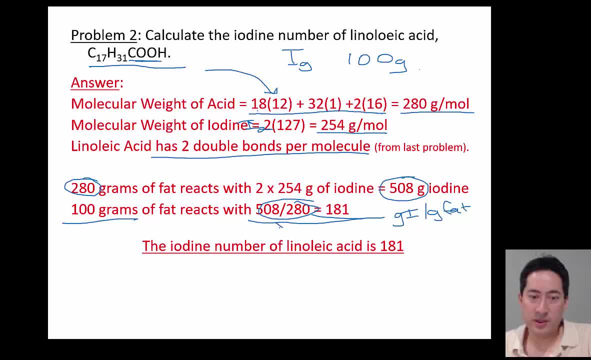 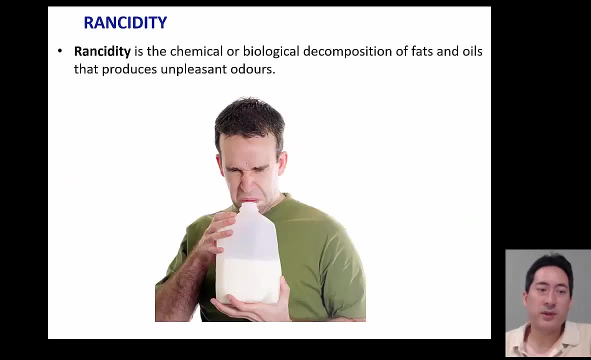 And so you need 100, so you actually need to times that. This should actually be times by 100 there, And so the number will be 181, which is Okay. All right, So Moving on. So fats break down in two different ways. 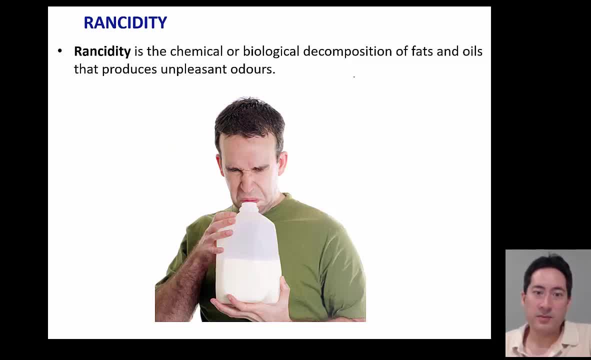 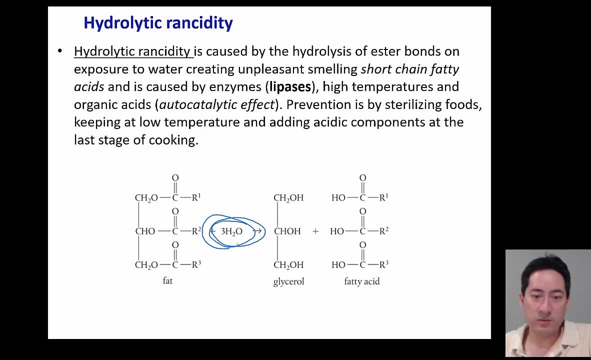 This is called rancidity And this is because this can happen, So there can be hydrolysis with water breaking it up. This can be accelerated by various things, such as enzymes, temperatures, organic acids, And the other way is oxidative. 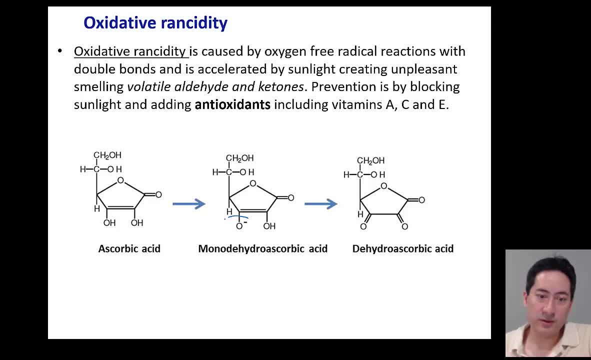 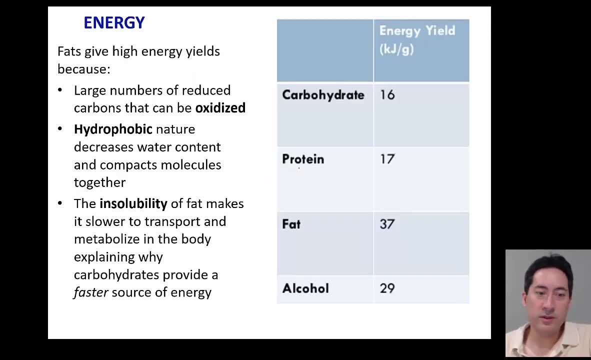 So oxygen, here that's a free radical and that's now formed a different chemical here, And so sunlight can accelerate these oxygen radicals coming in there and breaking down the fats, Moving on to the properties of fats. So properties Fats are very high. 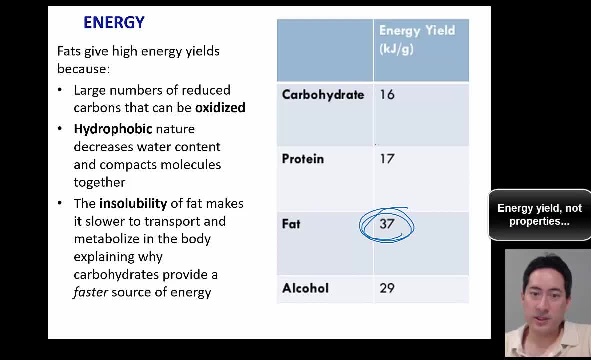 because carbohydrates and proteins. there are many, many oxygens, hydroxyl groups etc. coming off. these protein coming off the carbohydrates And proteins are the same, And so these fats have just completely reduced carbons covered in hydrogens. 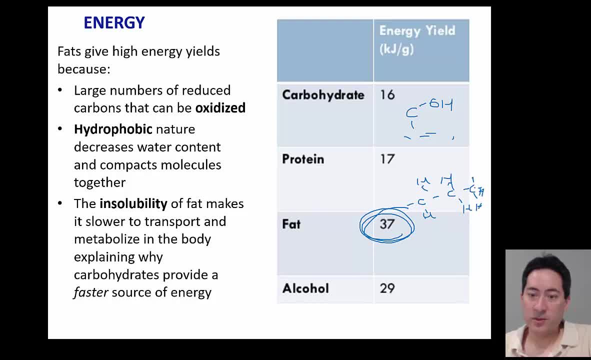 So there's a lot more. they're far more reduced. There's a lot more oxidation that can occur. That's why they produce a lot more energy. Second to that is they compact quite well together and exclude water, So it's a high density. 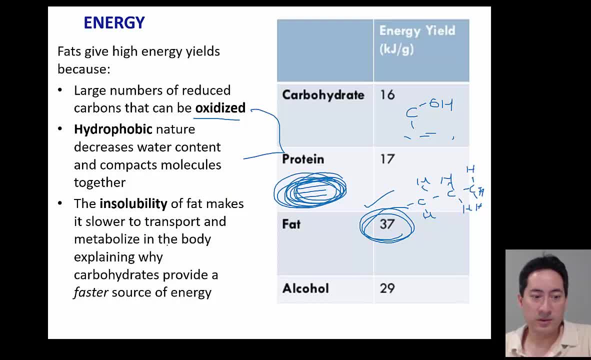 because they're hydrophobic. Insoluble is explaining to you, as I talked about in the previous slide, is why it takes longer to provide energy: because it's not soluble in water, so the enzymes can't get to it. So that should all make sense. 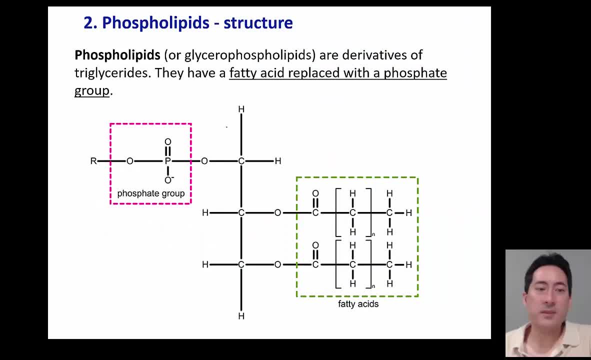 from what we've talked about previously. Okay, so the second major group are the phospholipids, which is basically what we've been talking about, but you get rid of on the carboxylic acids and add a phosphate group which is hydrophilic. 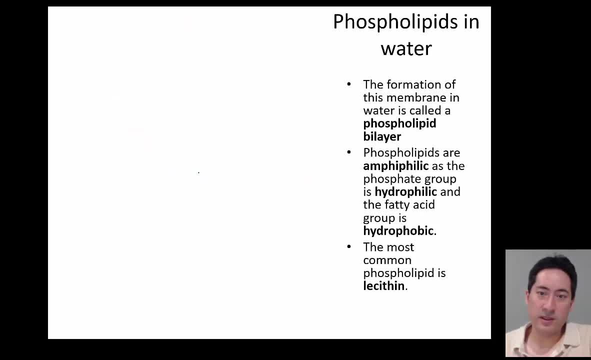 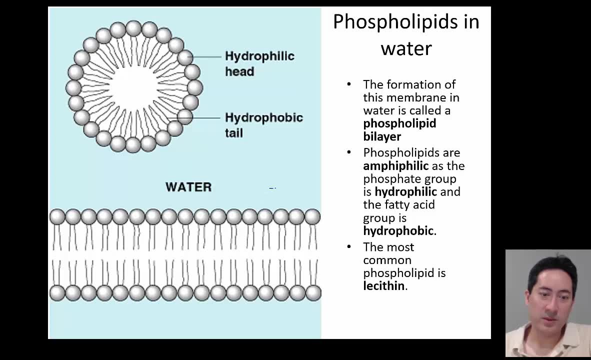 which is quite significant. So if you look at the uses of that, that is the cell membrane, And so that can be soluble in water and react with the water and then have this protective inside area That's hydrophobic, So that's called amphiphilic. 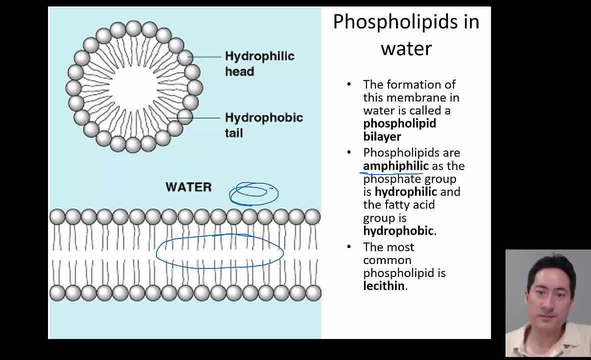 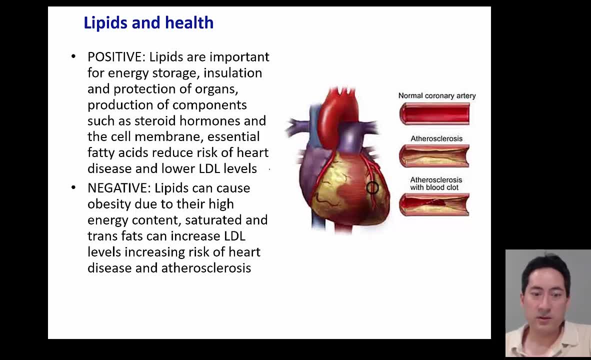 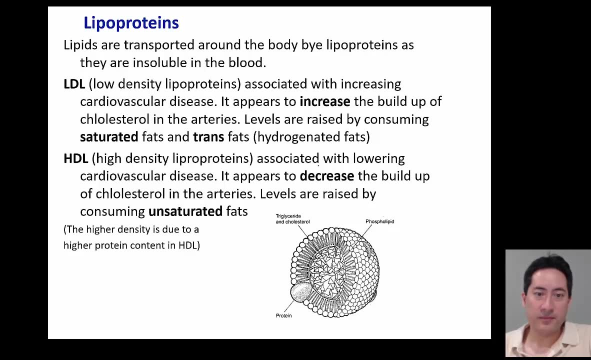 And we can move on. All right. so just going on to the health then. So the good, Let's just go to the next one. So the LDL, low density lipoproteins. So they are considered bad. They have lots of saturated fats. 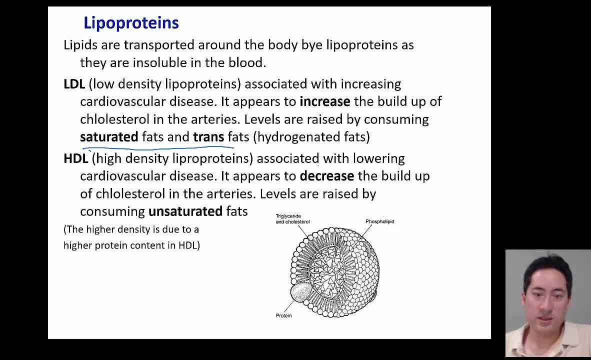 and trans fats. They have a lot of the high density proteins are considered good And they are high density not because they are unsaturated- Unsaturated is less dense- but because they contain these various proteins and stuff. So just high density is good. 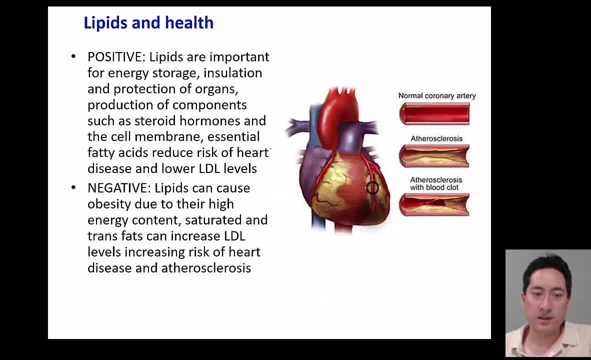 Low density is not good, So I don't know how much of this slide would be asked on a test. It's very much into biology now. So atherosclerosis, various heart disease problems, are all being linked with LDLs and HDLs. help rather than hurt. 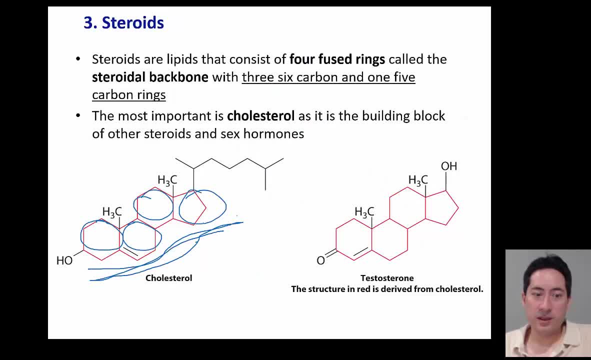 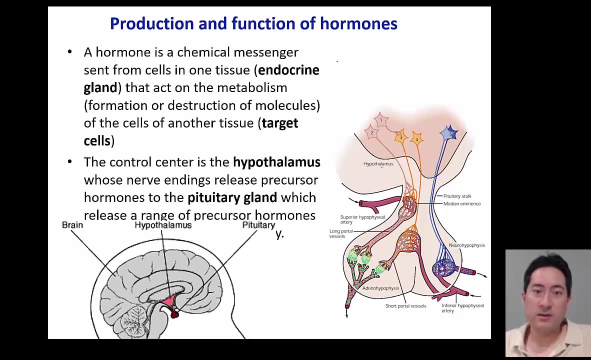 So I think we can move on to steroids now. So cholesterol is the main steroidal backbone and a lot of the other hormones in our bodies are derivatives of the cholesterol. So, moving back into biology here, I don't know if there's been an IB question on that before. 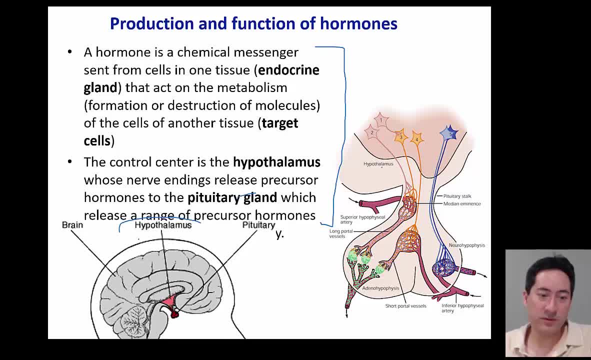 but just to quickly go over it, the hypothalamus is sort of the nerve interaction with the pituitary, And so there's the nervous and the hormonal systems that run the body, And this is where they link in together, And so the pituitary gland sends out precursor hormones. 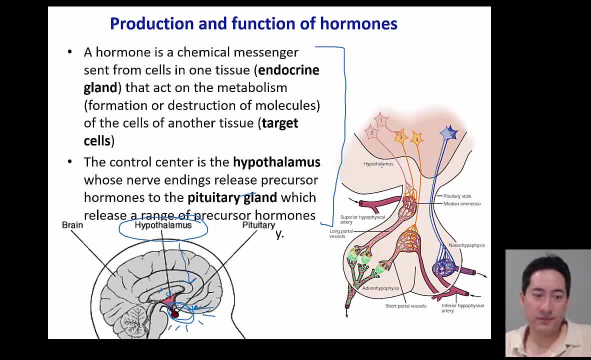 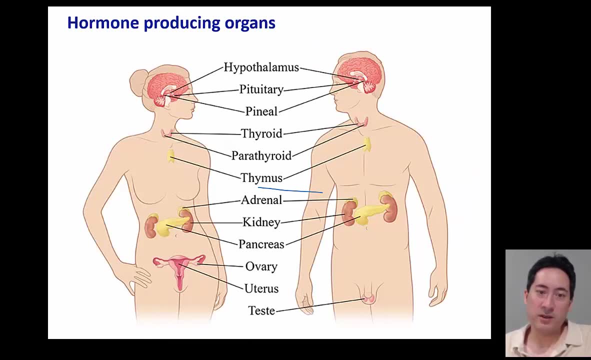 to all the other hormones. So it's right in the center of the brain and it's right in the center, That's where the two main systems of communication interact with the body. So that's quite interesting. So this quickly again, just to give you a quick overview.